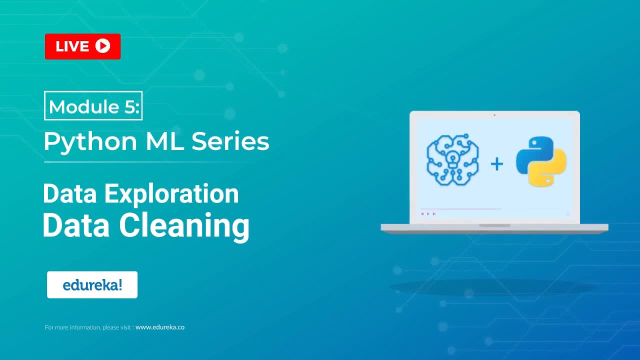 guys. and before we begin our session, let me just quickly get a confirmation, guys, if guys can hear me or not. So if I am audible to you guys, please type Yes in the chat box. And before we begin our session, let me just quickly get a confirmation, guys. 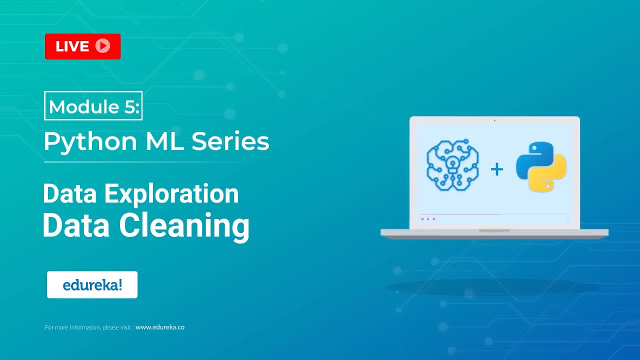 and now that I'm getting a lot of confirmation, Let's begin our session. guys, And if you are new here, don't forget to subscribe to Edureka for more exciting tutorials and press the bell icon to get the latest updates on Edureka and also check out Edureka's 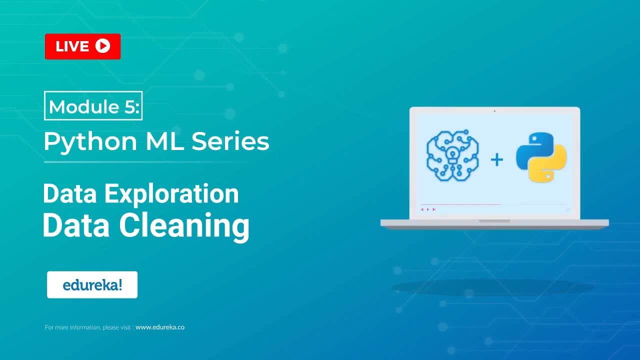 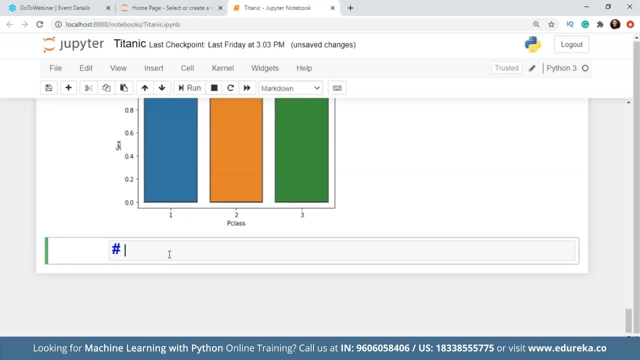 machine learning certification program. The link is given in the description box. All right, guys, so I'll just give it a heading. First of all, we are going to name this heading as cleaning the data. All right, So the very first thing. that, okay. 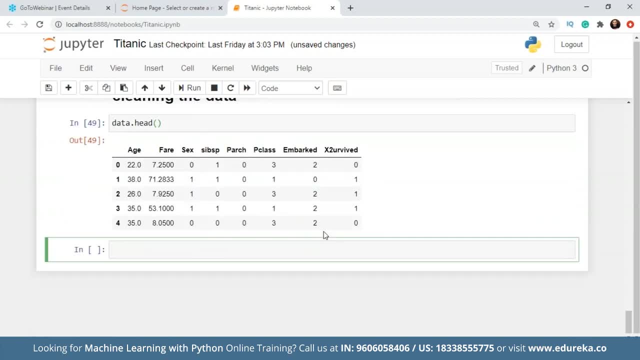 just get this data with top five rows. So we have age, we have fair, There is a gender: 0 is for male and one is for female. Then there is sibling spouses, children, The passenger class 1, 2 & 3, the embarked column. 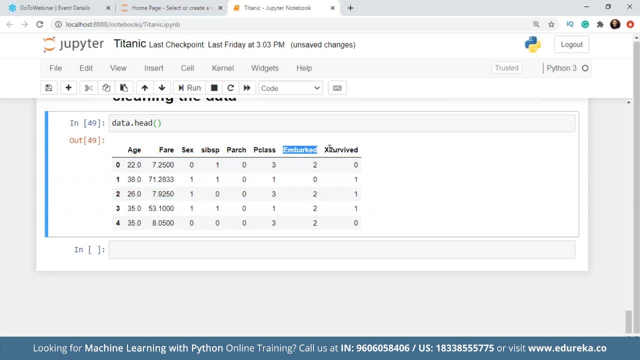 which has all the you know ports: Southampton, there's Queensland, There's one more, and the survived column, which is 0, is for did not survive and one is for survived. All right, so we know what our data looks like. now, The first thing that I want to check is: 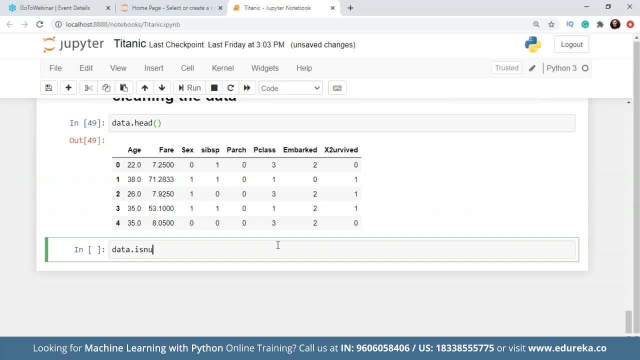 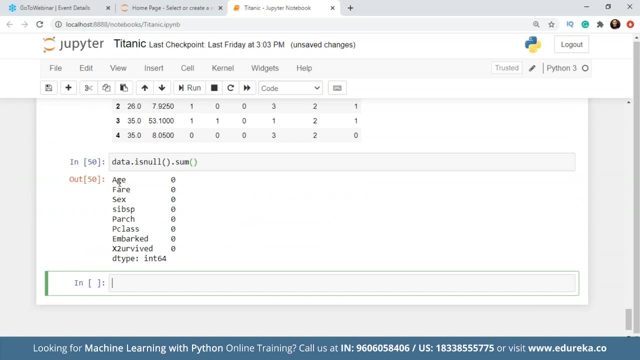 if there are any null values, guys. And if there are any null values, what I want to, I want to get the sum of all of them. So, since you can see there is no null value for any of the columns, because this data where we have downloaded it from. 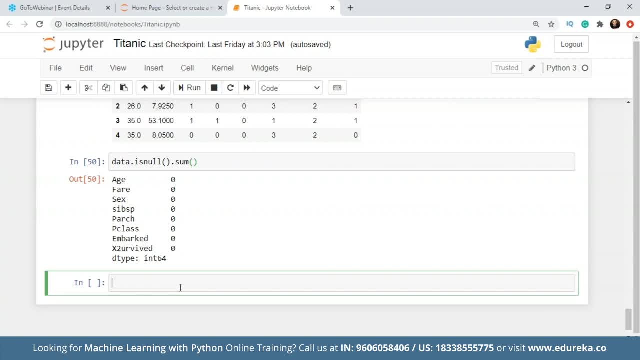 it's pretty clean, guys, All right. So what we know for sure is there is no null value, So we do not have to work on how we can get those values fixed. Let's take an instance where we say there is a few values here. 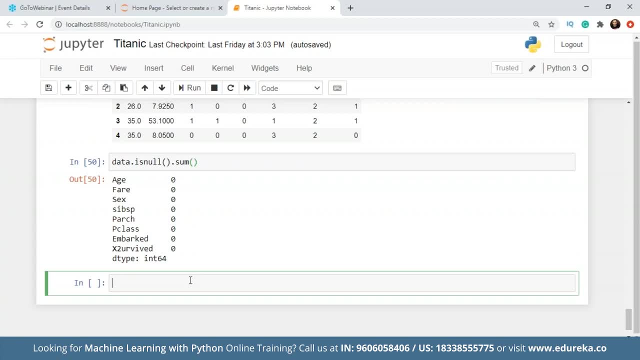 and there which are null value. So what we will do then? so the very first thing is, if the number of null values is pretty low, like out of 1300 values, only 70, or let's say 50, are null values. So what we could have done is we could have done data dot. 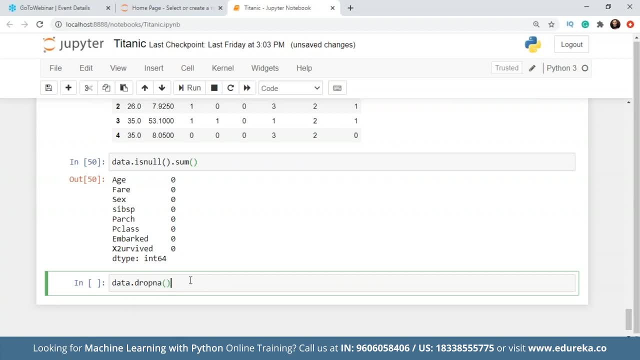 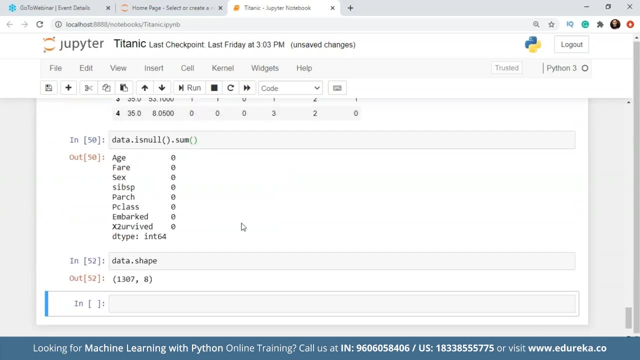 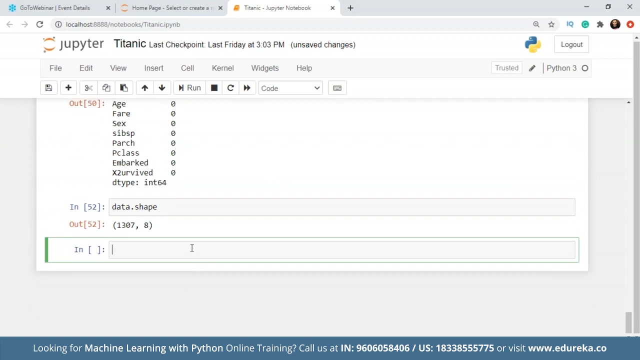 Drop any. that's it, Since we did not have anything at all, any null values. It did no change at all to our data, But in case if we had any null values, they would have been dropped. and one more thing: if we, there is a lot of null values that you have inside your data. 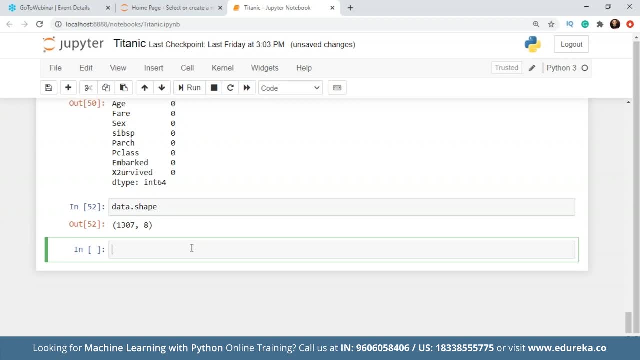 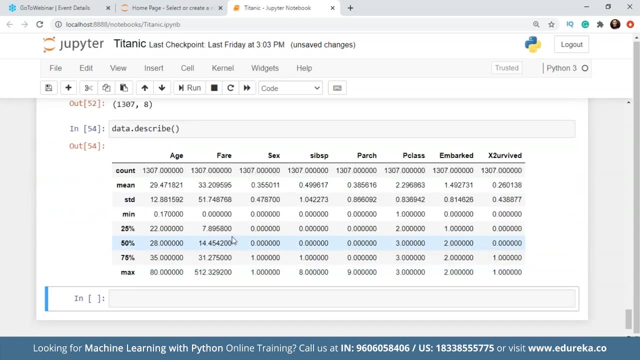 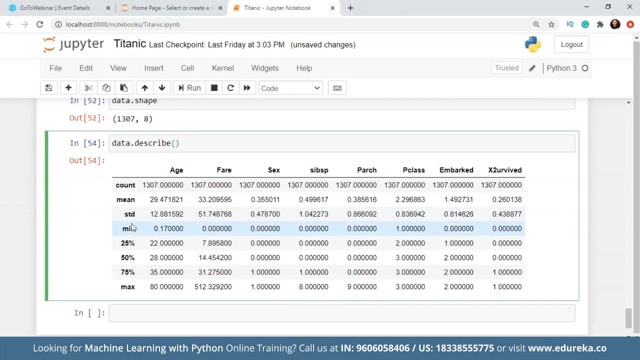 that is considered as noise, guys. So for that, what you can say, or what you can do, is get so one second, guys. Now the next good thing to do is fill the null values with an average, All right, so a median value. Let's imagine a scenario where we say: there is a ship. where is 1500 people? So what is the one thing that would not be clearer as in the era when Titanic was built, that is, 1919 or 1920s- late 1920s, We can say that- Or early 1930s? 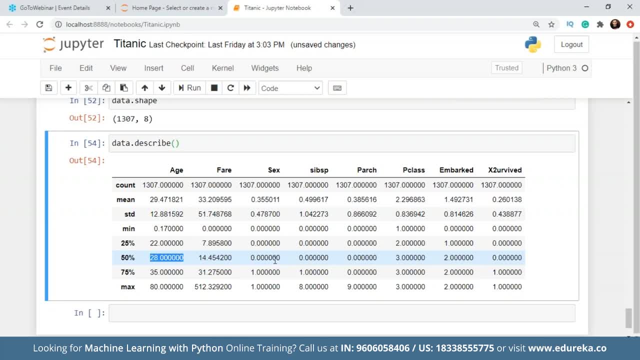 So I would say age would be a problem there. So let's imagine, like for age columns, We do not have a sufficient data. We have, let's say, 500 missing values. So what we can do now here is get a median which is 28 over here. 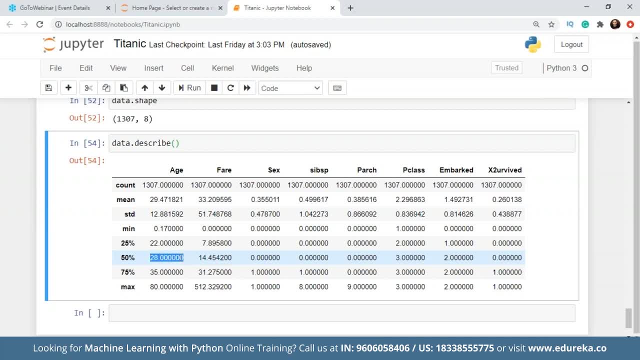 and replace all those null values with this value. So that is how we can do that and to do to do that, we can simply call the fill any method, That is, fill any and give it any values, since we do not have any values inside this. 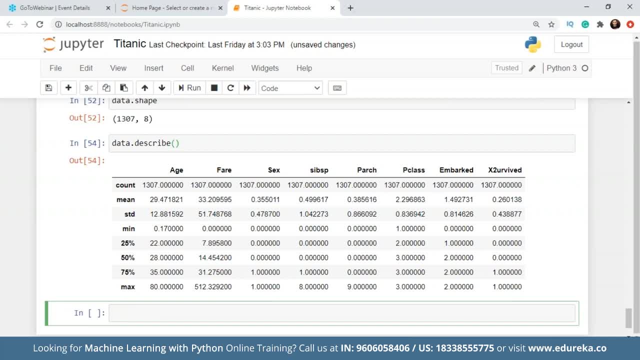 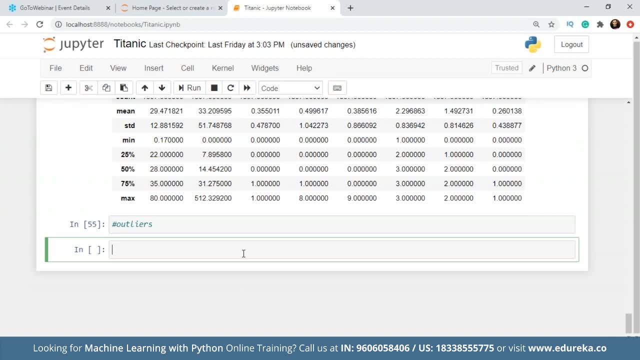 or so you don't have to worry about that. Okay, we'll move on to the next one, which is identifying the outliers. Okay, So what, basically, is an outlier? guys? an outlier is nothing but a value that is pretty distant from all the values. 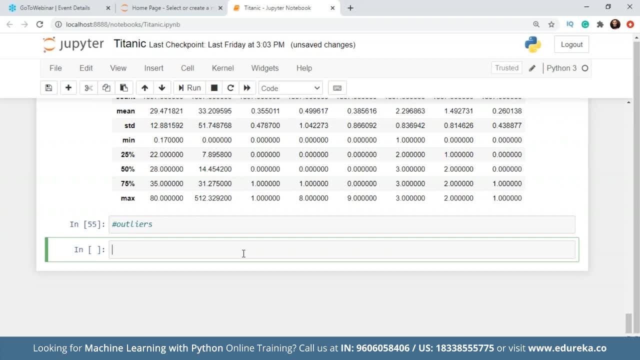 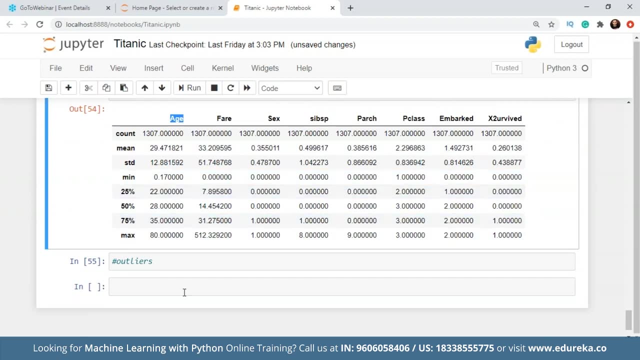 or we can also call it as an odd one out value. So let's say I have this column, Okay, This is a age called- and I'm seeing a lot of age- for let's say, there's a party somewhere and which is Millennial centric party. 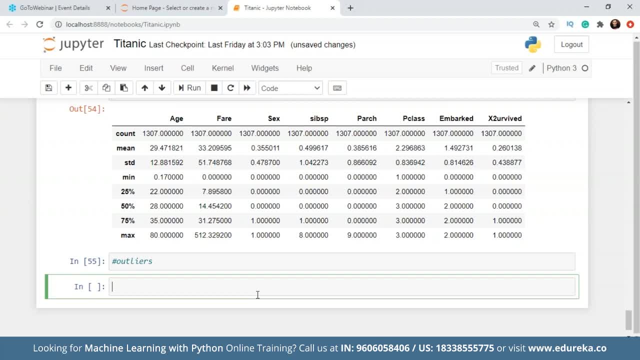 So it's got all the musicians and, you know, the rappers and DJs who are pretty famous in the Millennial population, but I'm seeing a lot of middle-aged men, women also enjoying there, which is not a bad thing, But what I would feel is that is a odd one out scenario. 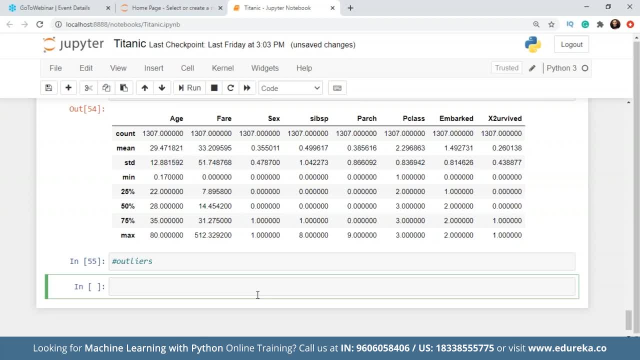 Similarly for outliers. Let's say, I have this age column and there are a lot of values between 30 to 40 years of age or 20 to 50 years of age, but I'm also seeing a lot of values which are 80, 92, 95. 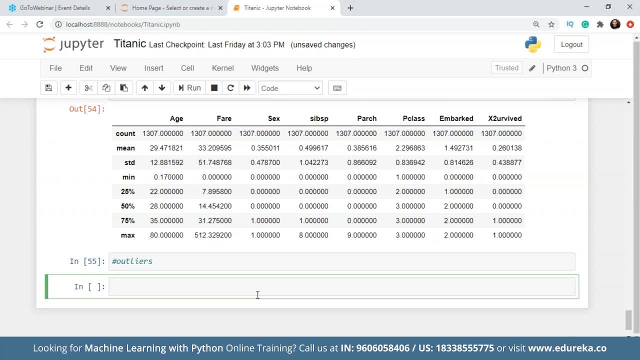 and some people over children whose age is 5, 6 or 7. So those are considered as outliers guys. So there is a way where you can find out. you know the outliers in your data. The very first thing that I also told you in the last session. 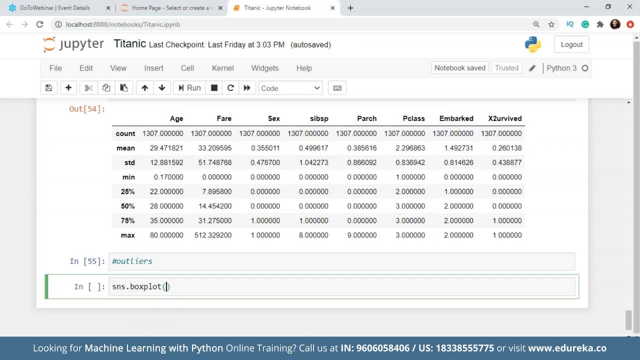 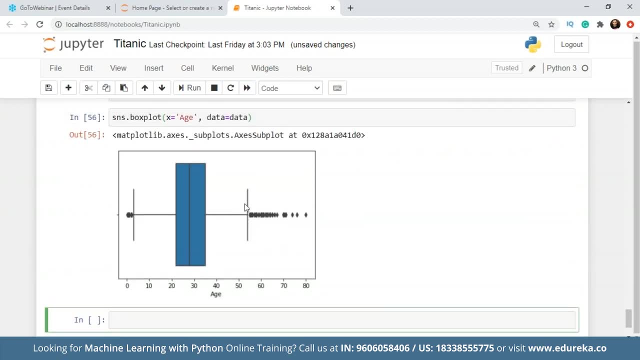 is how to count guys or box plot. So box plotting, Age data is equal to data. see: the data points after this point are considered as outliers and after this point also, it is considered as an outlier. This is very simplest, the simplest way to identify. 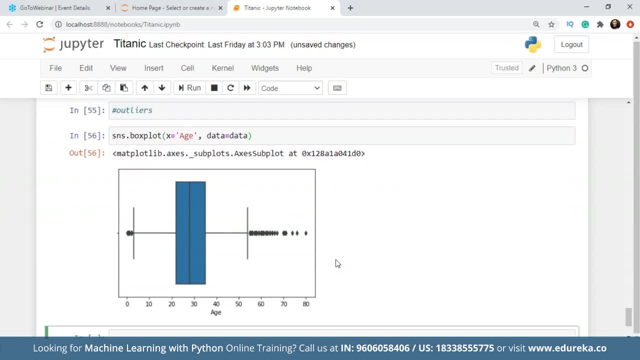 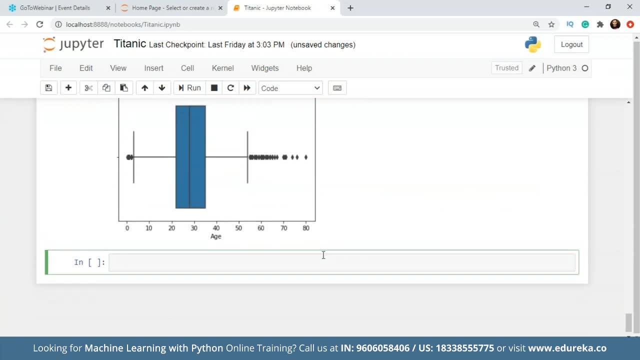 our outliers, since our data is pretty small and doesn't have a lot of entries. So it's good that we fix them by replacing them with a value, Or we could have also removed these outliers. There is one more way we can do that. 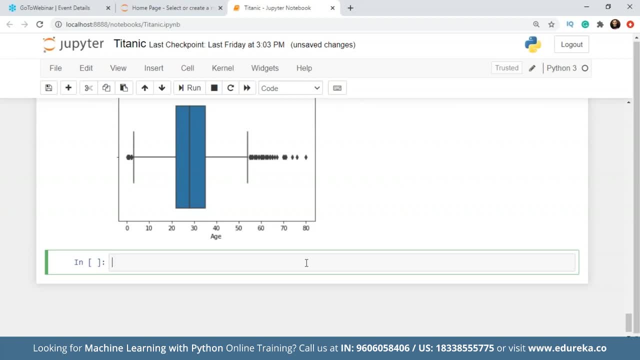 There is quantile data, dot, Quantile method, which you can apply for getting q1 and q3 values, which we can use for finding out the IQR. So you must be wondering what exactly is an IQR, right? Okay, So IQR is an interquantile range, guys. 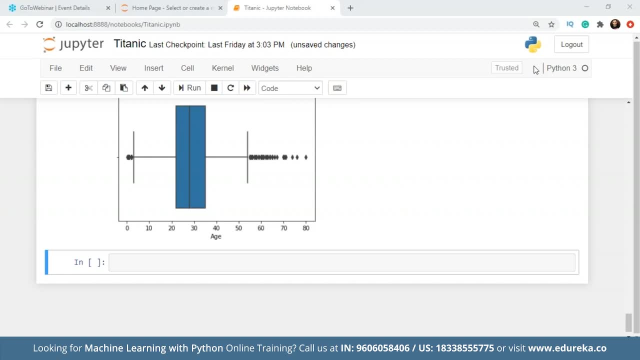 It's basically a measure of variability in your data. So, based on dividing a data set into quartiles, quartiles- I'm just told you that that is first, second and third. that is q1, q2 and q3 respectively. So now what we'll do here is we'll get the q1. 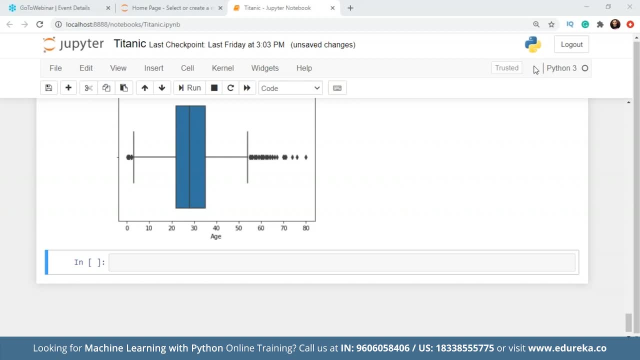 and q3 and we will have an IQR. Okay, All right, guys. So the very first thing that we would do, and we would get q1, which is all right. So let's print IQR, Data dot, Quantile, and I'll write a 0.25 over here. 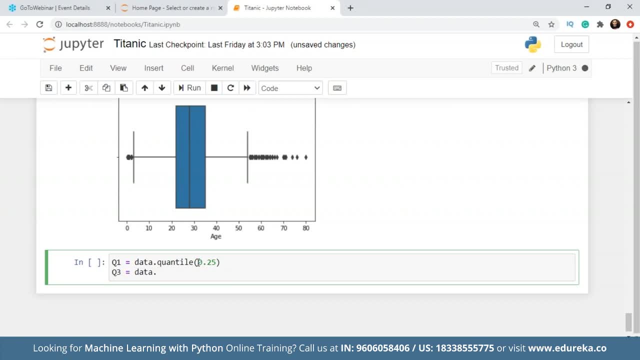 and q3 is equal to data dot Quantile, and I'll write 0.75 over here. and IQR is equal to q3 minus q1 and let's print IQR. All right, so we have the IQR for age, fair gender, siblings. 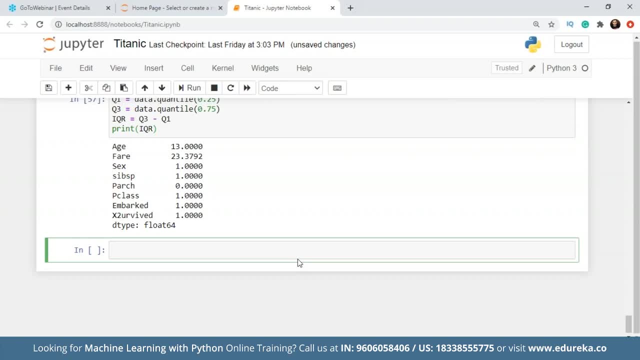 and spouses, children, passenger class, embarked column and survived. So this is the IQR that we have now to check how many outliers we have on our on our data. We will write it as data, So I've just copied this from the sample that I had made. 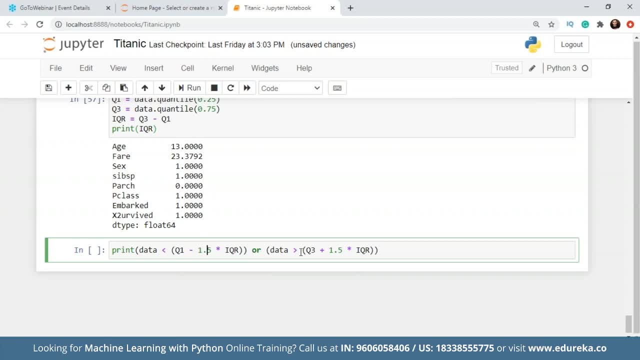 All right. So basically, I'll explain you what it is. So any data Point that is less than 1.5 x IQR or any data point that is greater than q3 plus 1.5 x IQR is considered as an outlier for us. 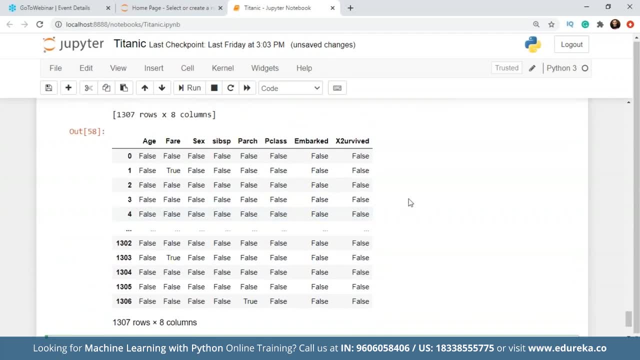 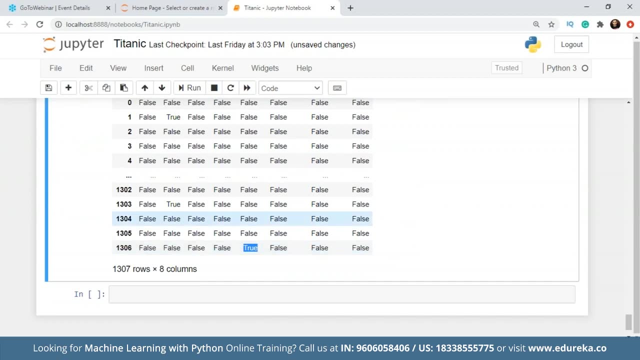 and for drastic changes or, you know, drastic data points, We can have one more value or it's. all these true values You see over here are basically outliers guys, So this you can find over here. So there are only a few values, Okay. 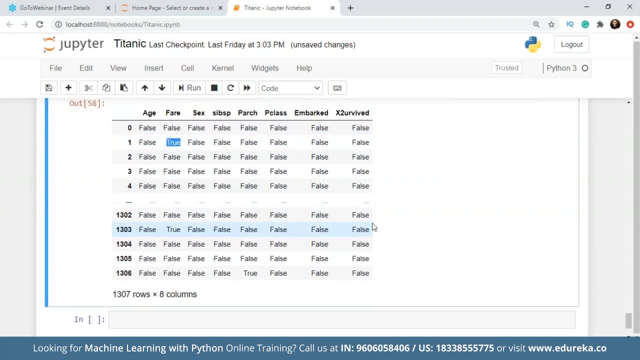 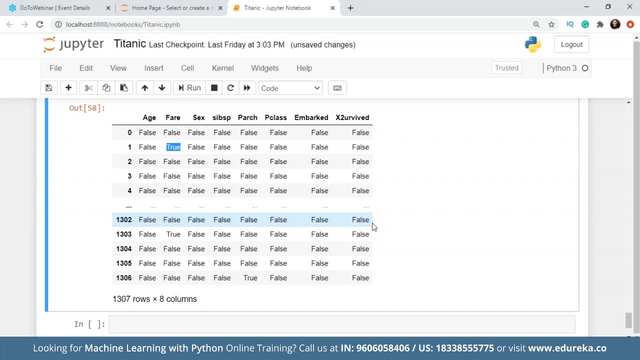 This is also an outlier, So we clearly have a few outliers. So what we can do now here is: I identified the outliers, So the next possible thing that we can do is we can get rid of them by removing them, but I don't want to do that. 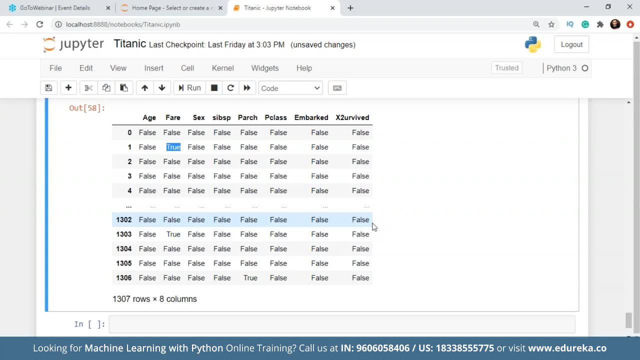 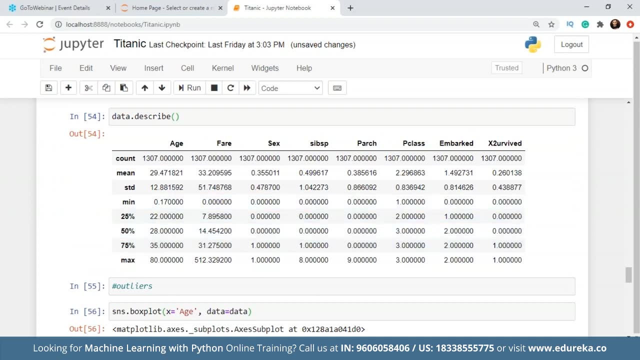 because that's a very easier option that we have. I want to replace it with: you know the median values, So we had the described column over here. I just quickly go back to it. So let's say, for fair, the 50% is 14.454. 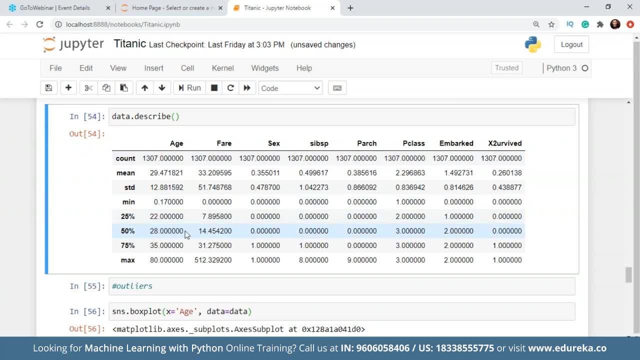 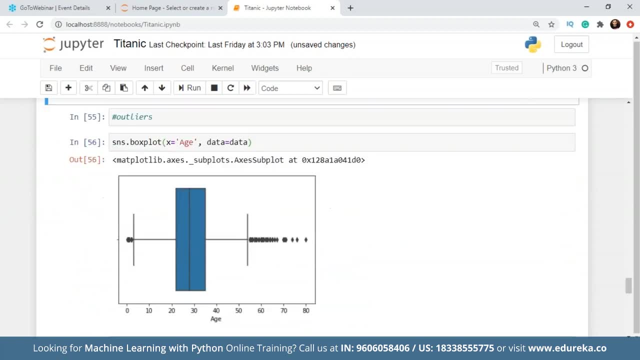 and for age It is 28.. So wherever we have found the outliers, I'm just going to replace it with these median values. So how would I do that, you ask? All right, So I'll tell you how to do that. 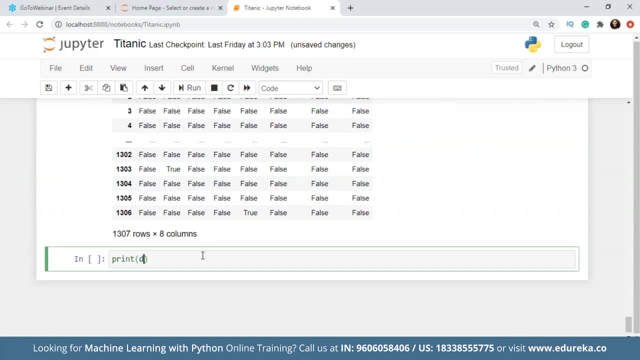 But I guess the first thing that I want to do is I want to check or print the Quantile value 0.5 for age column, And I'll also want to print data: age Quantile 0.95. Okay, wait a second guys. 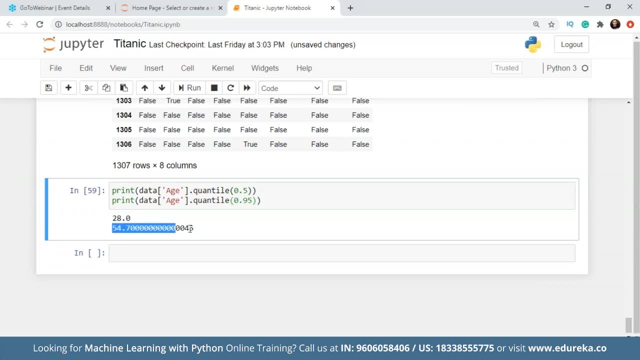 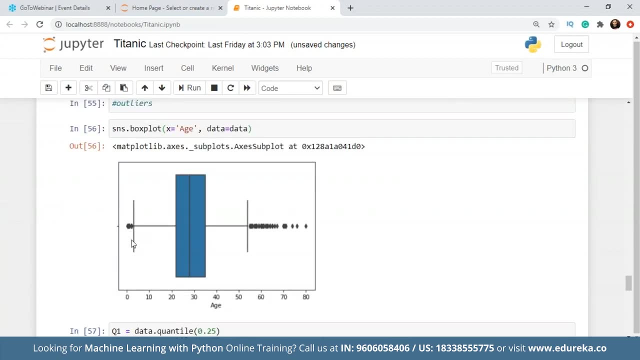 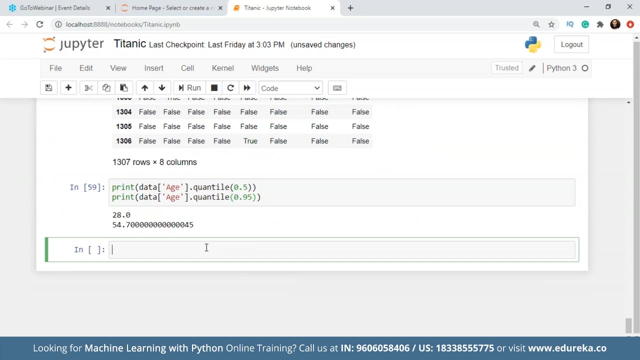 So we have 28 and for 54.. Okay, So let's just check the count, Lord, once again for age. So there are not enough outliers over here, And so we'll do one thing for every. All right, so we'll write it as: 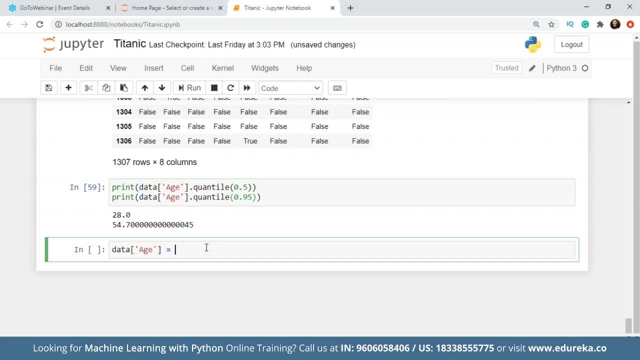 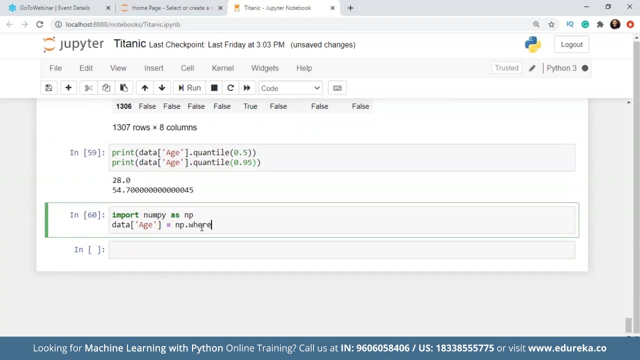 data age is equal to all right, We have to import numpy, and this is where all these are python libraries come from. It comes into picture, guys. All right, NP dot where data Age is less than call it 15, or we don't have want to actually do that because 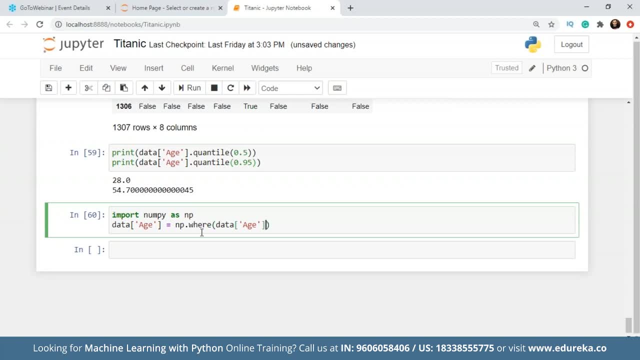 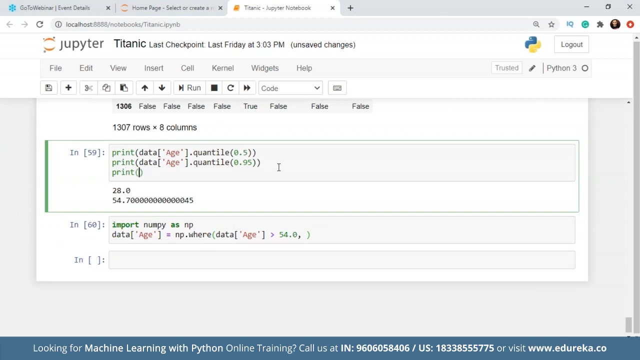 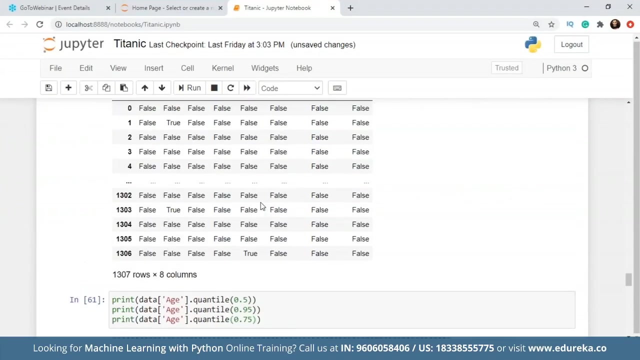 these are 0.5. Quantile is actually 28.. So we'll do it only for the age that is greater than 54. point 0 will replace it with some value, which is going to be, let's say, if you're getting an error. 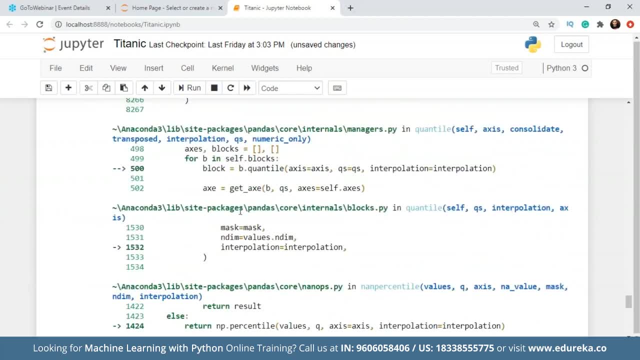 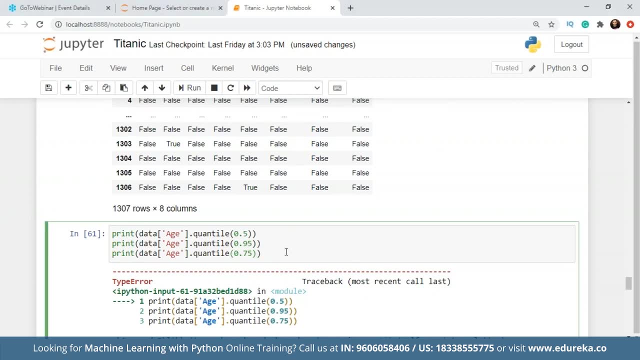 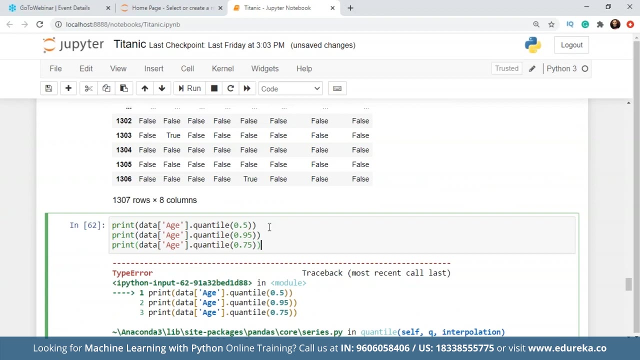 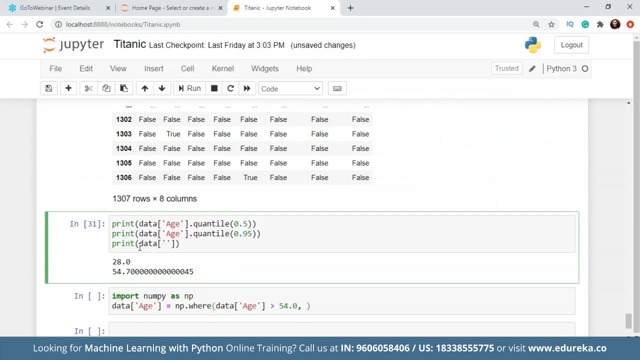 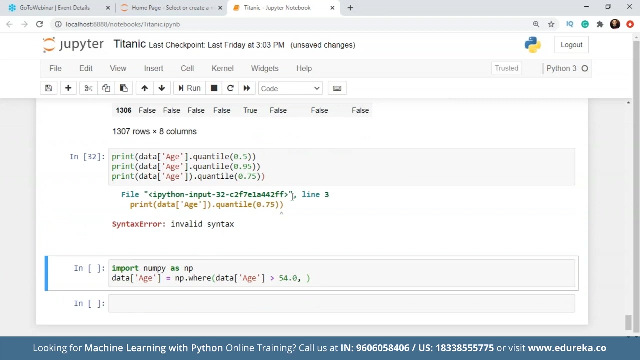 why are we actually getting an arrow? Okay, wait a second, guys. All right guys, so let's print that value. I ran the shell again and Okay, guys, Quantile, and we get this 0.75 value. We have an invalid syntax. 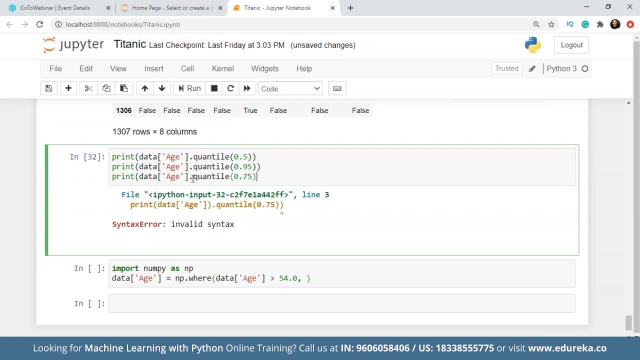 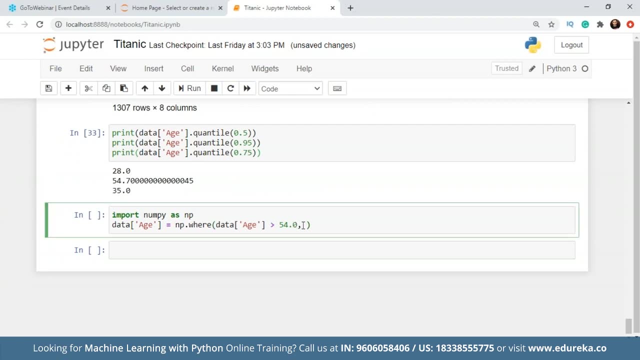 All right. So there you go, Just 35. All right, So what I'm going to do is, for every value that is greater than 54. I'm going to replace it with, let's say, 35, and data is equal to data. 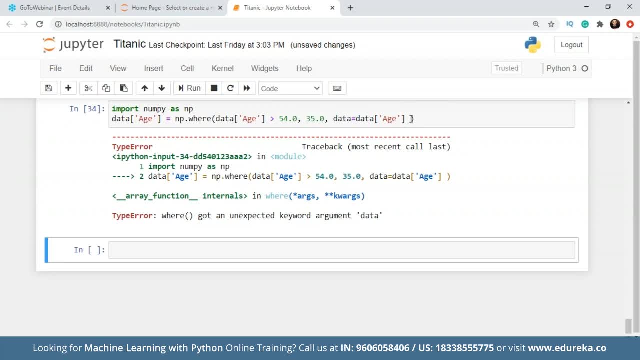 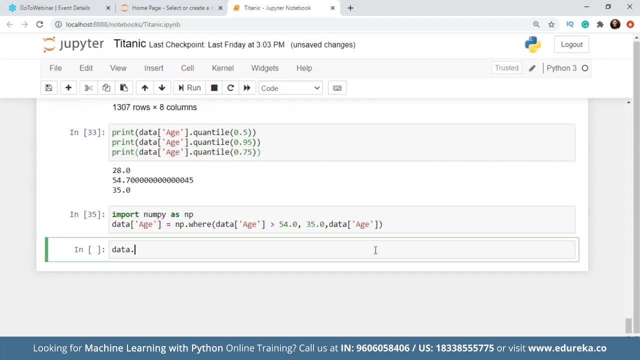 age. Okay, All right guys. so I don't think we have to mention data over here. We can just go with this, All right. So now what I'm going to do is I will check What is the highest value that I have. 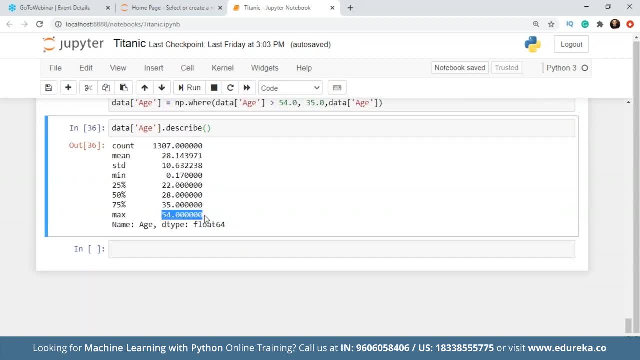 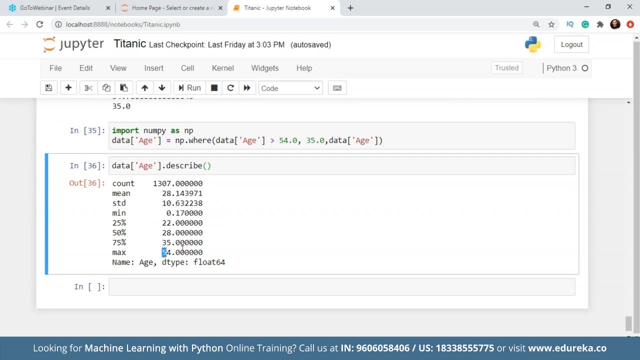 It's clearly 54 because we have stopped it at that. So after 54, we don't have any values. So any value that is above 54 or more than 54, it's going to be replaced with 35.. So that is how you replace values in your outliers, guys. 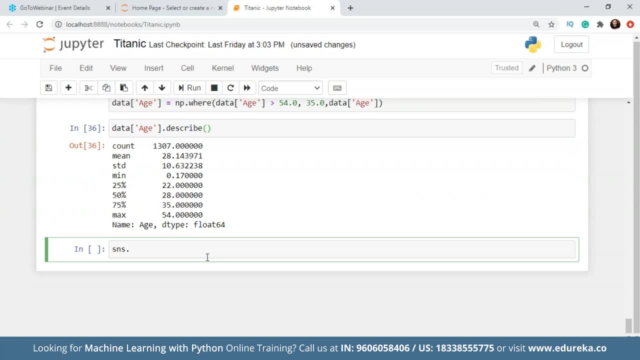 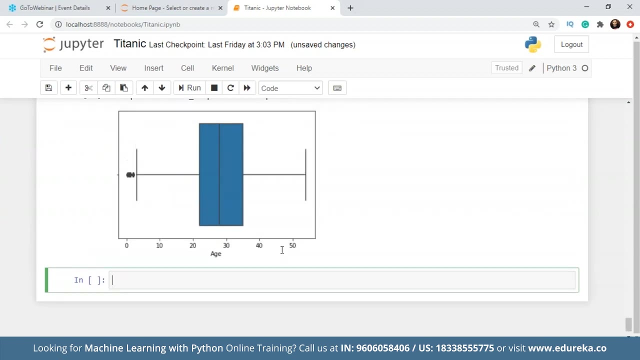 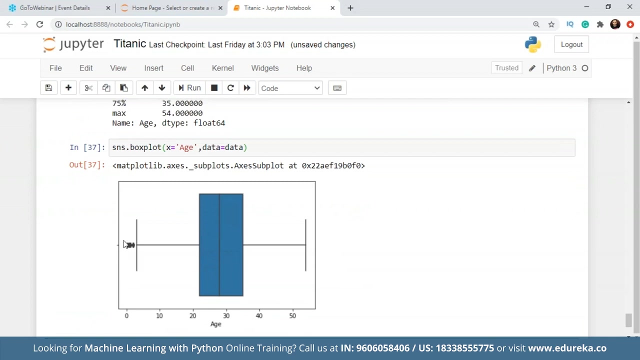 So now I also you can check for a box plot, So you will see a lot of outliers must have gone missing. As you can see, guys, all the outliers, they that over after 54 are missing, and these are a few more outliers that we have. 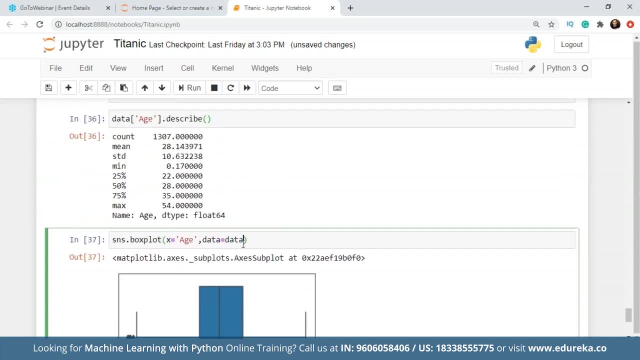 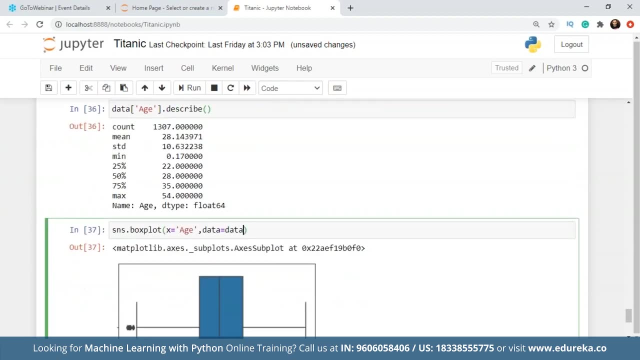 which I'm not actually removing, because you don't have to remove all the outliers guys. Sometimes they can be useful. Sometimes you remove all the outliers, It affects your model as well, And similarly for other columns that may face a lot of outliers. 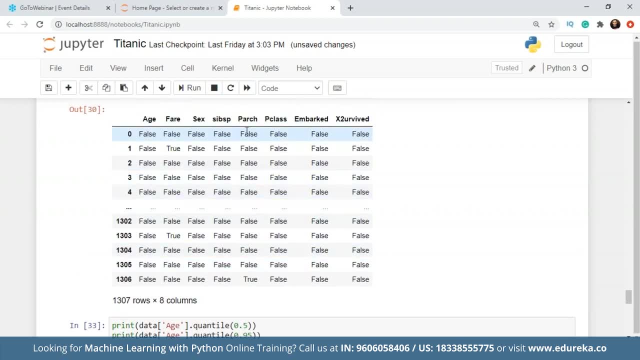 So we did it for age. I can see there are a lot of for children and for siblings and spouses, and if you take a look at this one, which is fair, So there is also a lot of outliers for fair as well. So let's do it for fair. 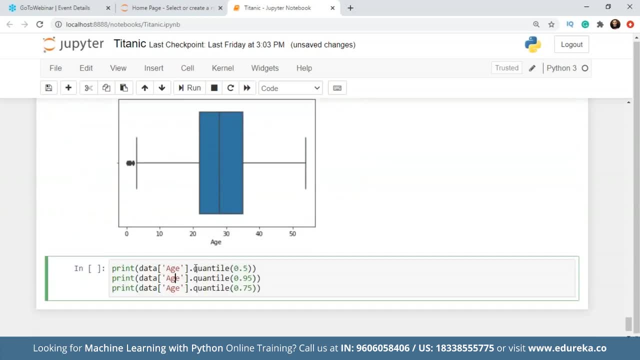 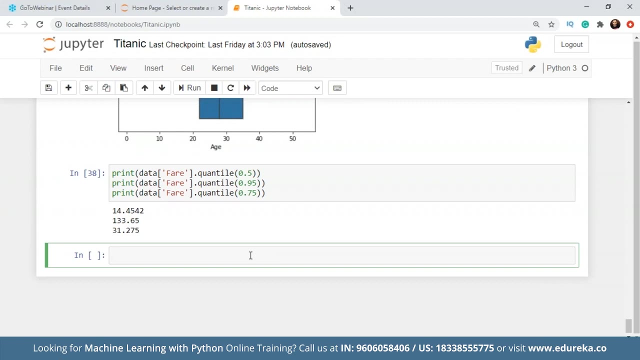 So I'll just copy this code and instead of fair: Okay. Okay, there are a few problems here, guys. So even if I remove, okay, let's get a box plot for fair and we'll see You know the most number of outliers lying. 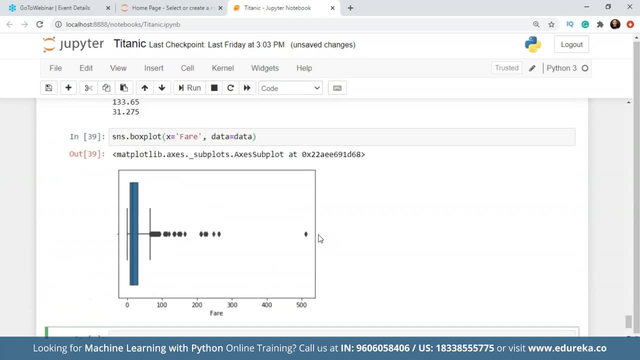 in which direction that we should remove. So after 100, there are a lot of outliers, guys. So this is because we are seeing this spike or we are doing these outliers, because there are a lot of passengers in the non-surviving area who paid less for a fair. 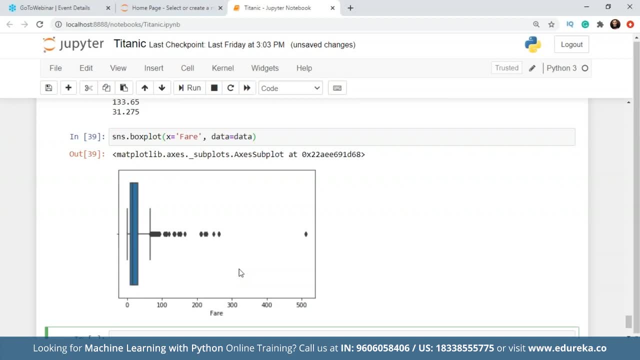 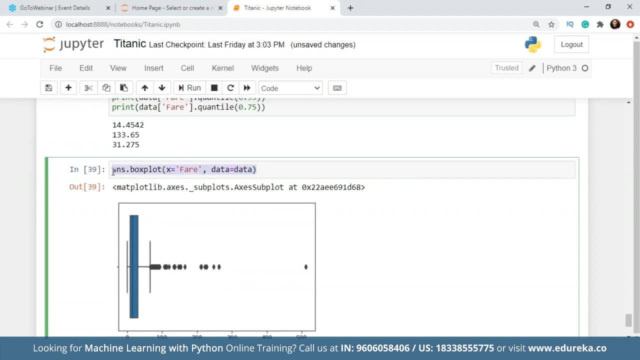 and there are a lot of people who survived, who paid a lot more for fair and also survived the shipwreck. So we will not replace these values with anything because these are important for the model. instead, What we'll do will create a different groups. 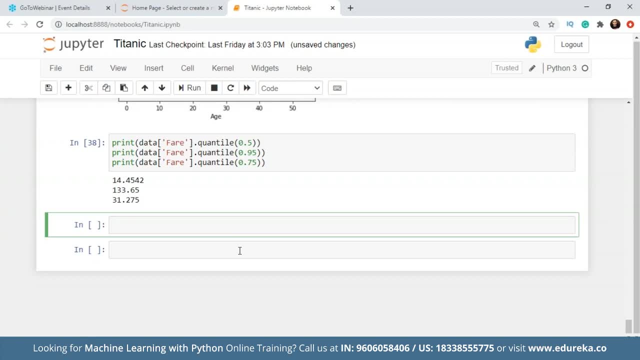 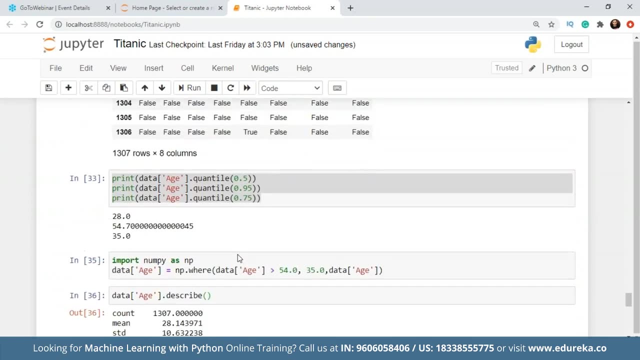 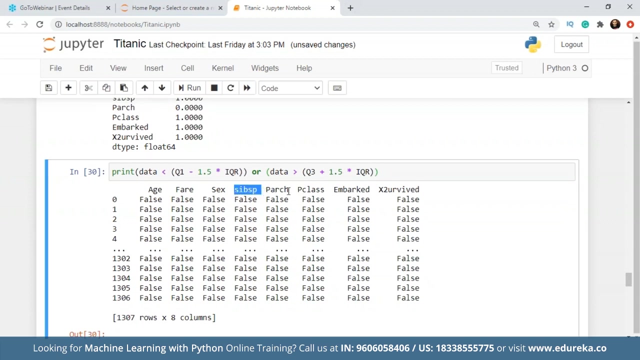 in the later on section, which is feature engineering. So, as far as cleaning the data is concerned, that is how you do it guys. So we have done it for the fair and similarly for other columns. like children, The siblings will create a one column altogether. 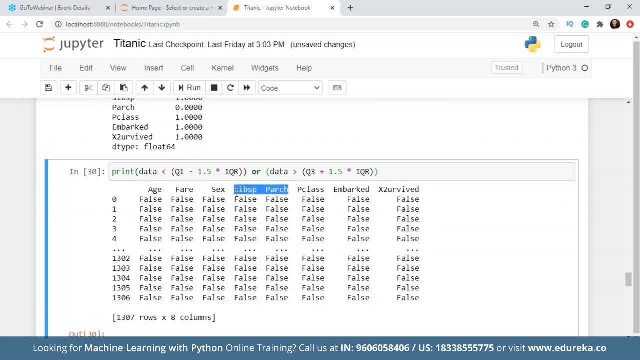 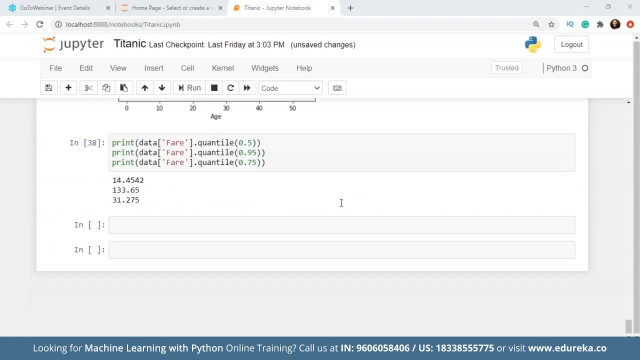 which will have a company or sort of, or you know. you know if you had any family, so we'll keep one or zero for that. That is also known as a feature engineering, or we can also call it as one hot encoding method, and now that we are done with this session, also. 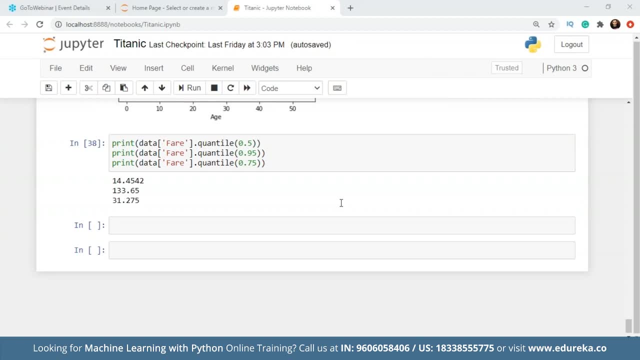 So I have told you how we can clean our data by removing outliers. There are other ways also that you can do that, But this is the simplest way I can find for the beginners. It's quite easy, guys, Also, if you clean your data well. 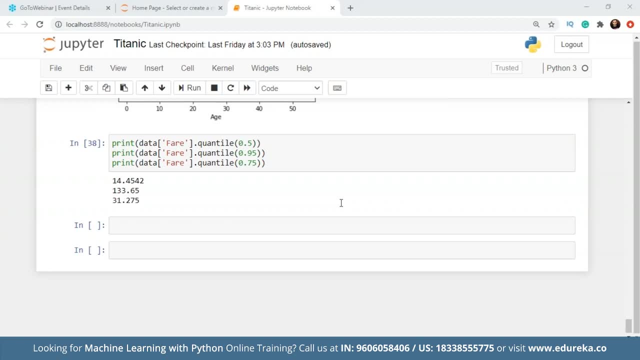 you remove the noise, which eventually helps you in getting across, or you know it helps you in avoiding overfitting and underfitting. So I'll just quickly tell you what exactly is overfitting and you'll get a greater idea of what exactly is go fitting. 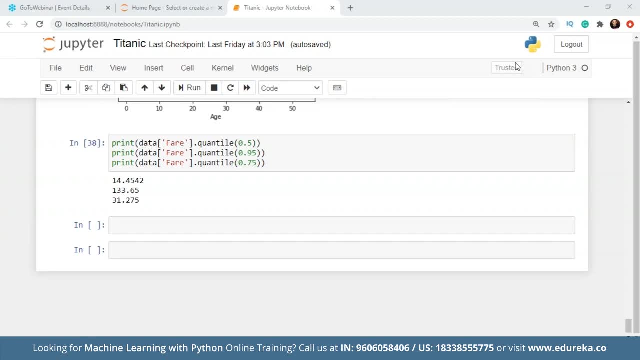 So noise is basically that data that is irrelevant for our model. So, similarly, if we look at our data, so there are a few columns that you can drop before We're feeding it to the model for the training data. So I'll just quickly tell you what exactly is overfitting. 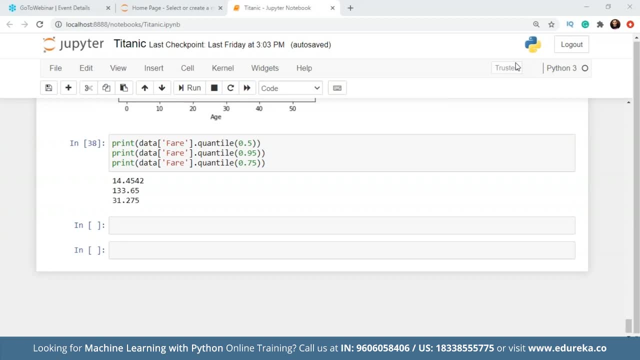 So any model is said to be overfitted when we feed it a lot more data than necessary. All right, so to make it relatable, you can imagine trying to fit into our size apparel or any clothing you know. if it's oversized you will not make it a good fit. 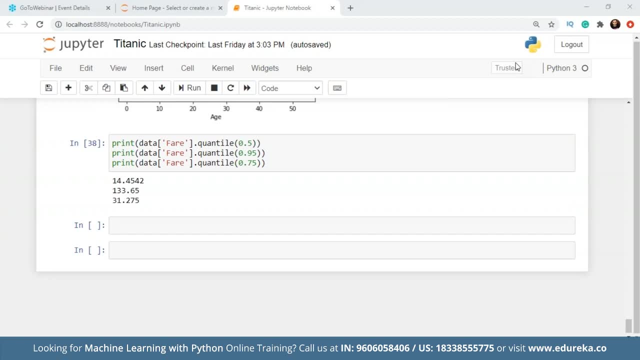 So that's also known as overfitting, where we're giving it a lot more data than it actually needs, and that lot more data includes the noise and the irrelevant redundancy of the data. So if you are reducing or removing this noisy data and all those redundant variables or columns, 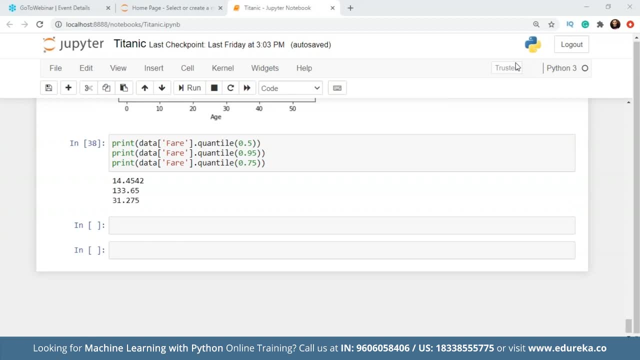 you're actually making the fit quite good. If you're able to overcome this problem of overfitting, your model will be a quite good guys. and we'll be talking about cross validation, So we'll know about variance and bias. Also, if you are not feeding your model enough, your model 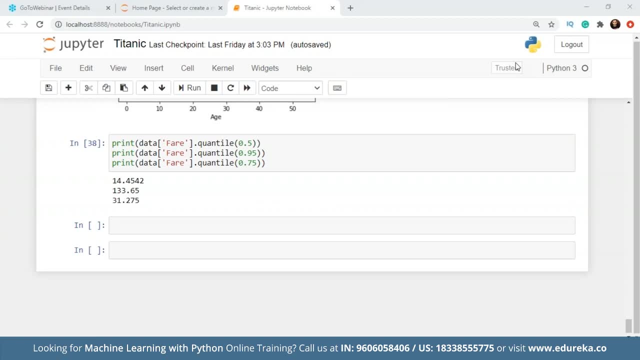 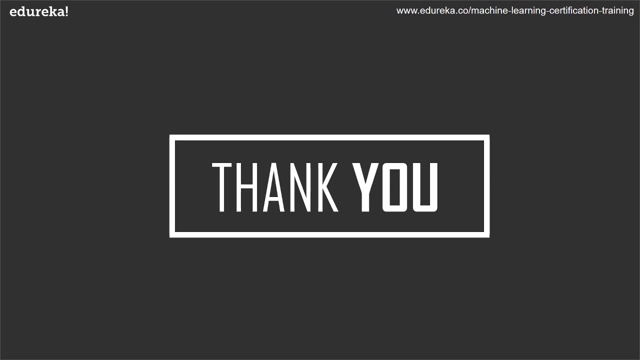 also gets an under fitted guys. So that's also one way to do it. but to avoid overfitting in machine learning or to avoid under fitting in machine learning, We have several values or several methods. So we have cross validation. We can do cross validation to do that. 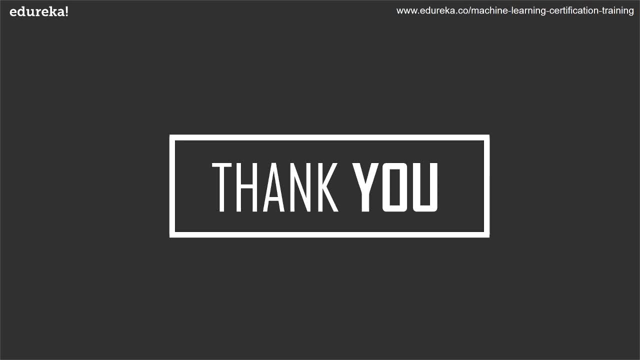 There is a. we can train it with more data. with more relevant data, We can remove redundant features. There is a regularization and assembling. All right. with this, we have come to the end of the session, guys, and tomorrow at 10 am We are going to resume with the session 6. 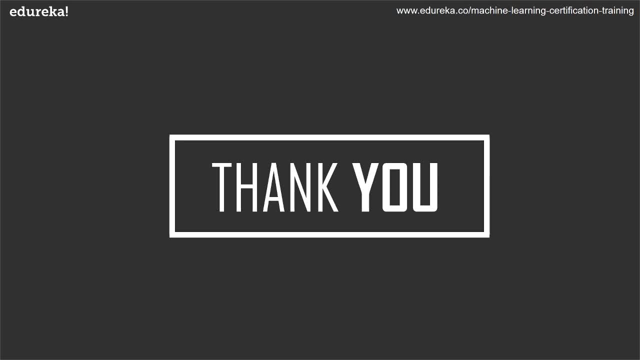 where we are going to do the feature engineering. and for these five sessions I want to give you an exercise to complete, guys. So make sure, whatever data that you're using, make sure there is no null values in over there. and see you, guys, in the next session, guys. 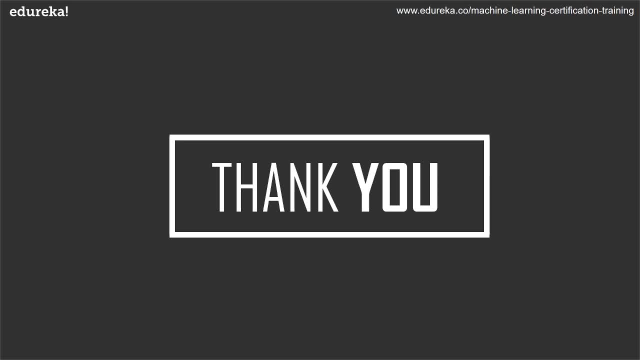 And if you're new here, don't forget to subscribe to your data car for more exciting tutorials and press the bell icon to get the latest updates on a direct call. and one more thing, guys, If you are looking for a machine learning certification program, 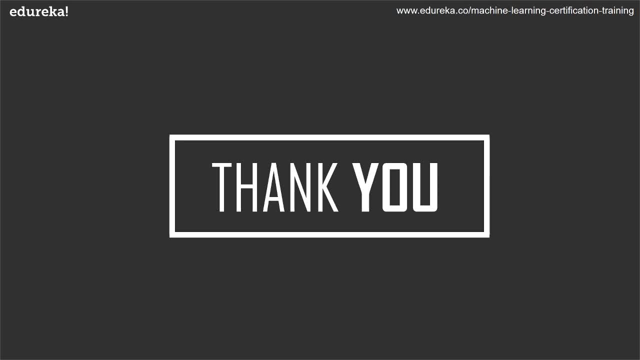 there is a link in the description box below, So go there, check it out, and I'm going to see you in the next video. See you in the next session, guys, So have a nice day, Thank you, Thank you.